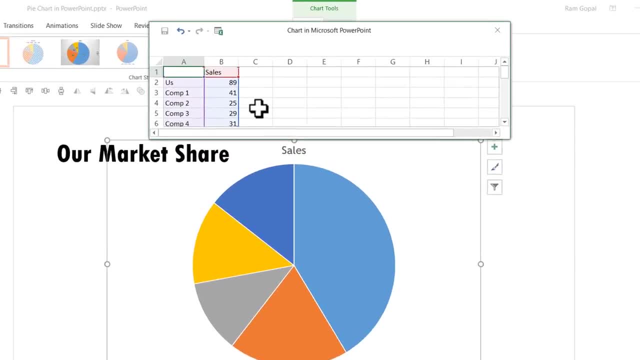 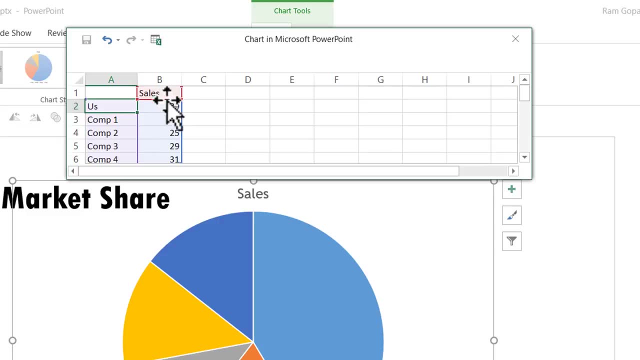 And, yes, I have replaced the sample data with my own data And here it shows our performance compared to four other competitors And the values are shown in this right hand side And I have given the header as Sales And I am going to close this particular worksheet. 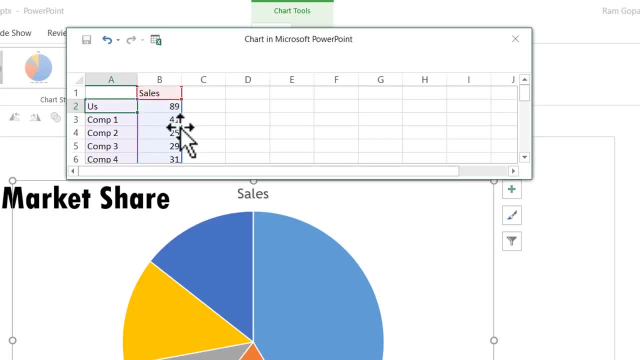 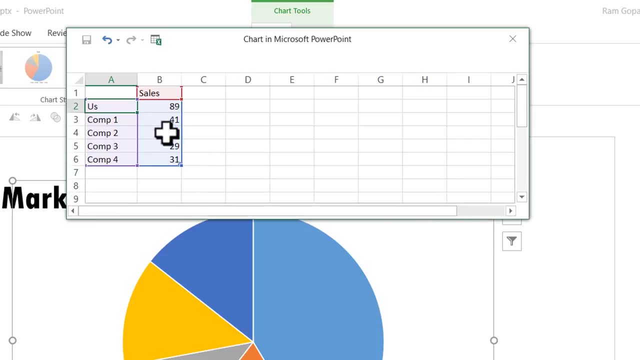 And, as I mentioned in my earlier videos, if you want to see more of the sales, you just need to move your cursor To the bottom right corner of this worksheet And you can click and drag so you can see more of the data. 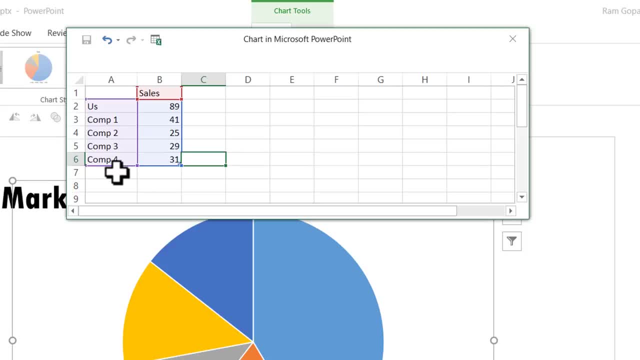 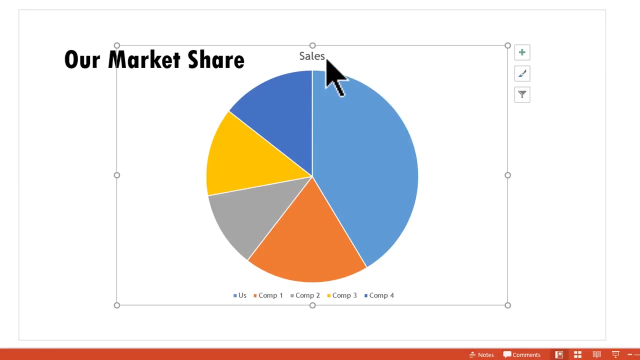 And if you want to add more category names, you can always add here And then populate with corresponding values And the selection will automatically include those as well. Now let me close this worksheet, And now we have the chart here. I typically prefer to have my chart title as my slide title. 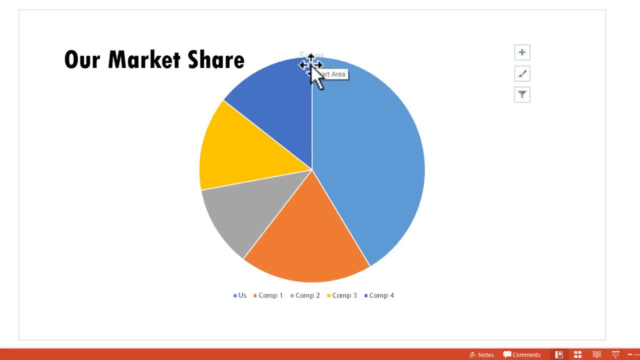 So I am going to select this chart title And I am going to press Delete So I don't have the chart title there. I am going to resize this by holding the Shift button down. as I click and drag from the corner, As I reduce the size, you can see that the chart is now of a much better size. 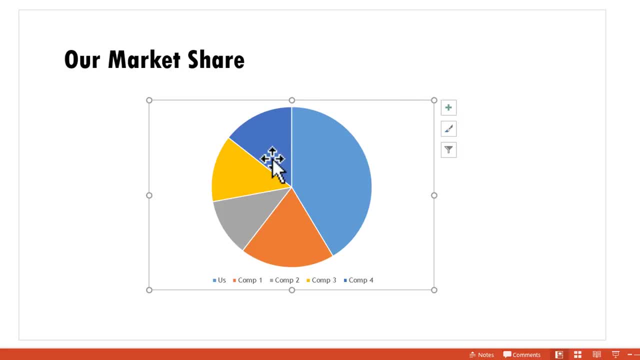 The next thing is, as I resized this chart, you can see that the font is not very easy for people to read. So I am going to click on the bounding box outside And then I am going to go to Home tab And I am going to increase the font size. 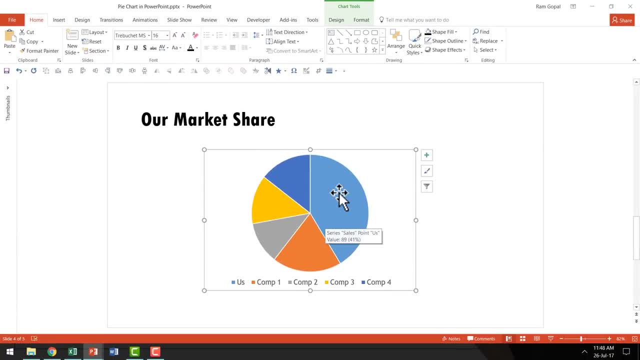 So that it's much easier for people to read. And this is how a typical pie chart looks. Now there are a few things that we can do to make this chart a little more easy to understand for the audience. The first one is by adding data labels. 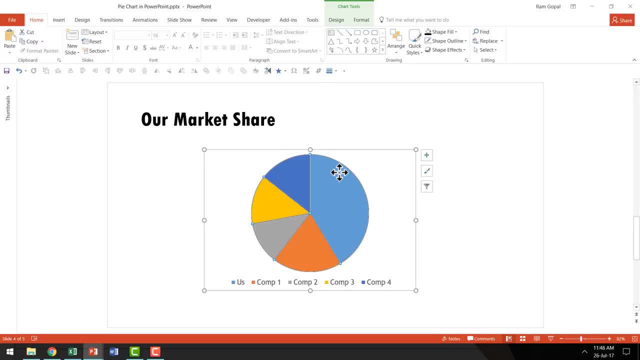 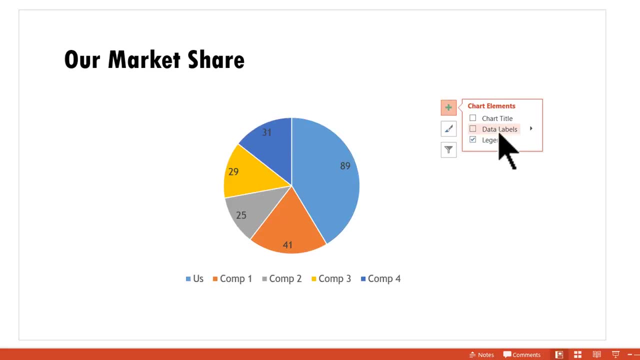 Now what we are going to do is I am going to select the chart here And then you can go to the option here called Plus, which is about the chart elements, And here you see that there is this option called Data Labels. You can click on the small arrow here to expand where exactly you want the data labels to be. 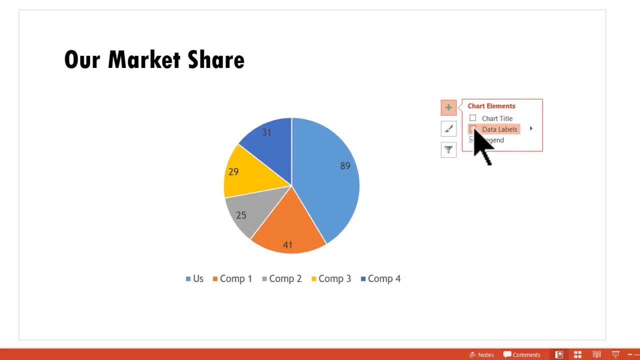 I am not really going to go into all those elements, I am just going to say Tick, and here my data values are populated. Then I am going to click on this once again so that I don't have that fly out menu. And this is now a much better chart, because the values are very clearly shown. 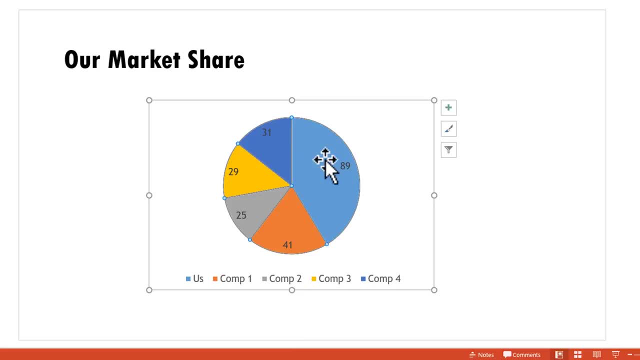 And the next thing is to make these data labels easier for the audience to read. Sometimes there may not be sufficient contrast between the font color and the background color. In this case, you can see that the background color is dark blue and the font color is black. 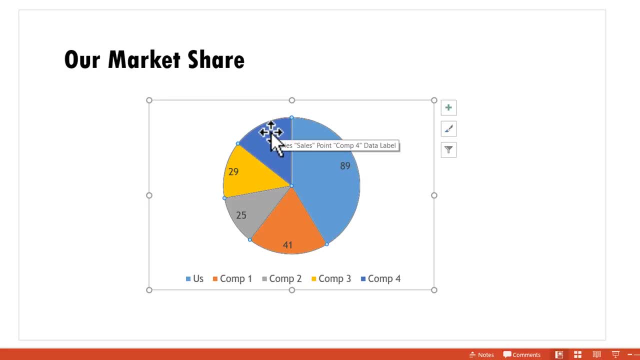 So it is not very easy for the audience to read this value. So I am going to click on the data label. On the first click, all the data labels are selected. Then I click on the same data label once more and that selects only that specific data label. 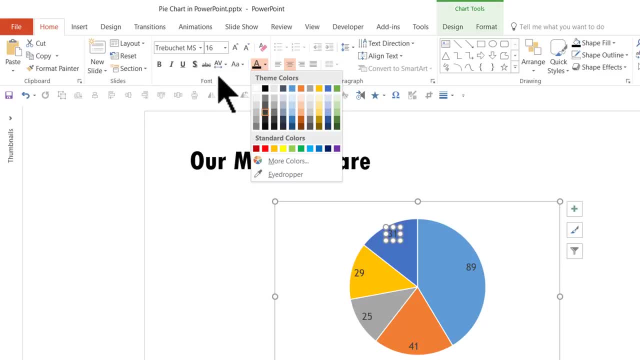 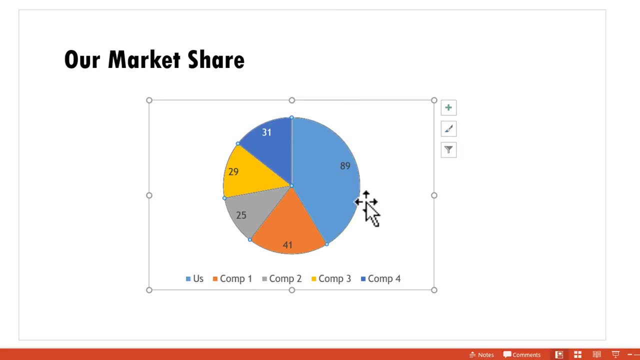 I can go to the Font group here in Home tab, And then I can go to the Font group here in Home tab, Then change it to say white, and now it is much easier for the audience to read. And now this chart is a little better. 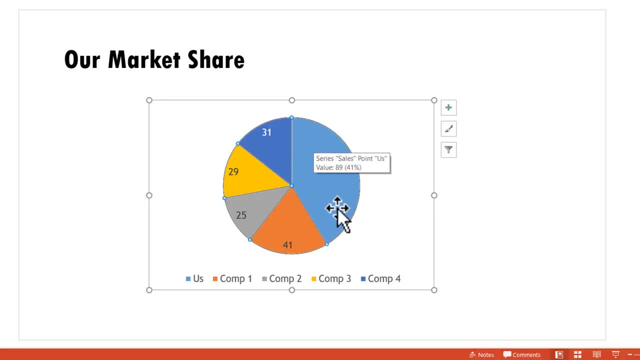 Then I want to show my performance a lot significantly compared to the others. So I am going to first select this segment alone. Now you can see that the entire pie chart is selected. Then, when I select this particular segment alone, you see that when I click on it, only this segment is selected. 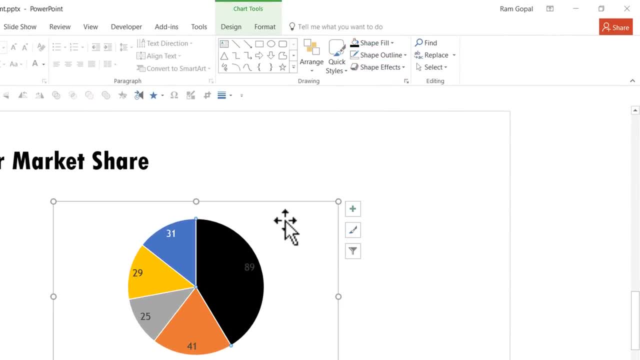 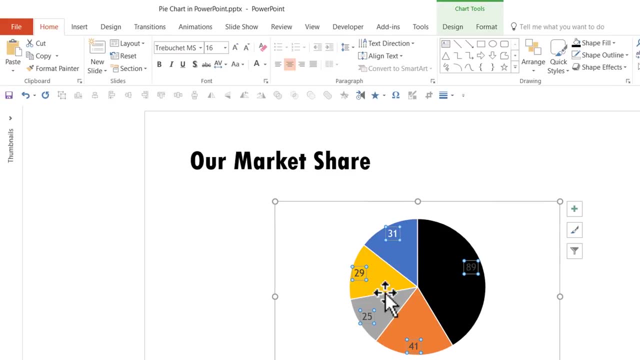 I am going to go to Shape Fill and choose- maybe black, Which clearly stands out from the rest of the colors, And I am going to do the same thing for the data label as well. On the first click, all the data labels are selected. 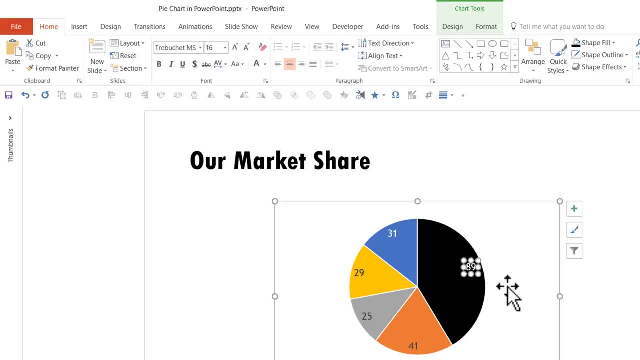 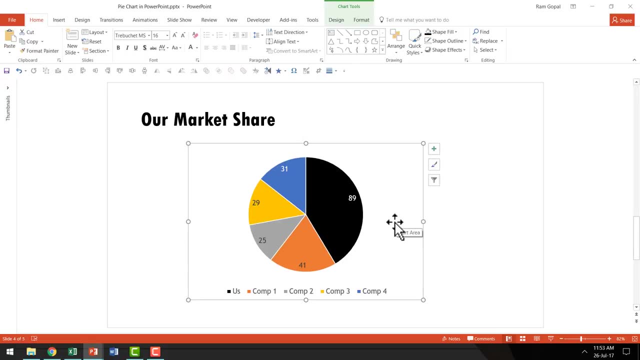 Then I click on the specific data label and make it white, And now this chart is way better than what we have started out with. The next thing we are going to do is to make this chart into a donut chart. A donut chart is considered as visually more interesting than a typical pie chart. 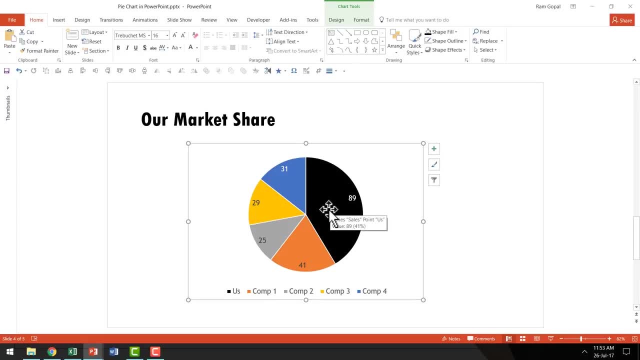 And it is very easy for you to convert your pie chart into a donut chart. After all, it is another chart type of the same category, So I am going to select the chart here And then go to the Design tab in PowerPoint ribbon. 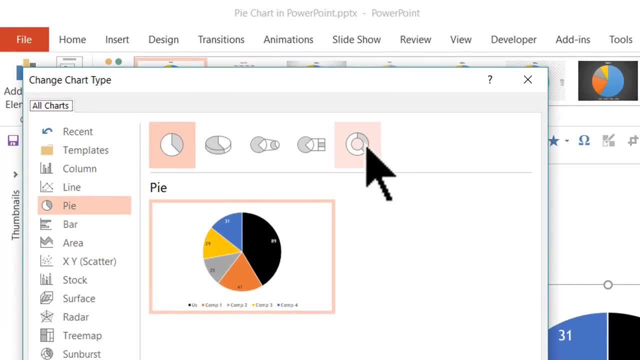 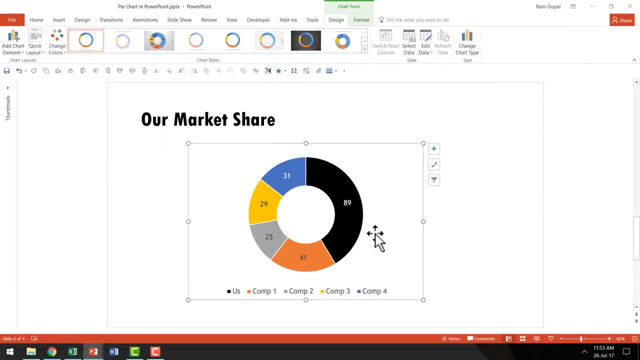 Go to Change Chart Type option And here you see that we have donut chart available here And you click on the donut chart and you say OK, And instantly your pie chart is converted into a donut chart. Now you see that these kind of charts are used in infographics, in financial magazines, in newspapers etc.